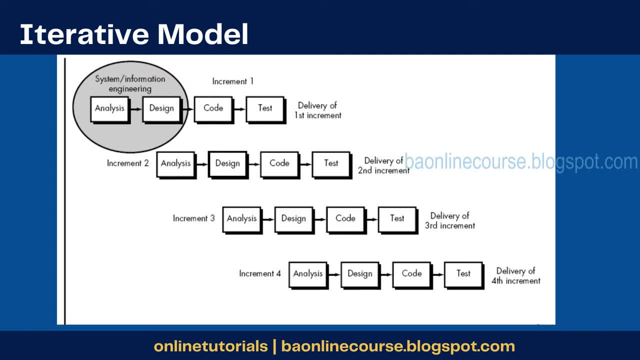 Why the gamut to cover. But you know, if you want something specific- I don't know- I can provide you some high-level view of documents, which you can do Because you know, even if I would have to say I would cover banking that has so many you know. 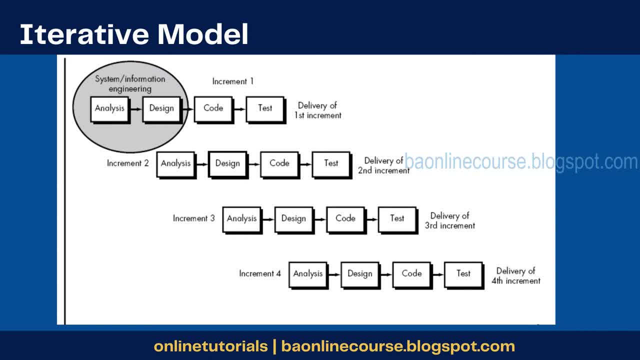 Right sub-topics within it. it would be impossible to be covering it in one or two sessions, even 30 or 40 sessions, Okay. So, whatever the use, okay so whatever the user stories, you would be focusing mainly on which kind of domain to have a good knowledge on it. 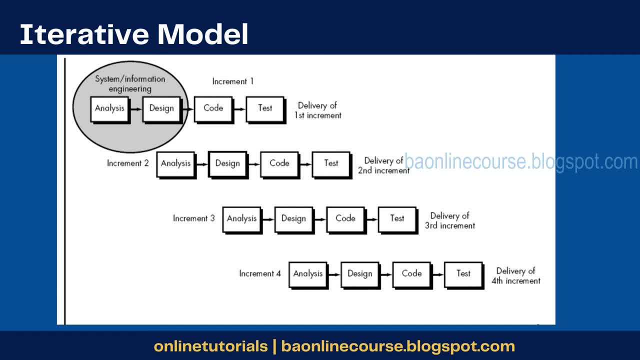 We will take example. We will take examples for when we are covering those topics. so we will cover both the use cases which are UML-based, which you typically do it in a traditional SDLC, and user stories, when you are doing it in an agile way. right, so both of them would be covered. yeah. 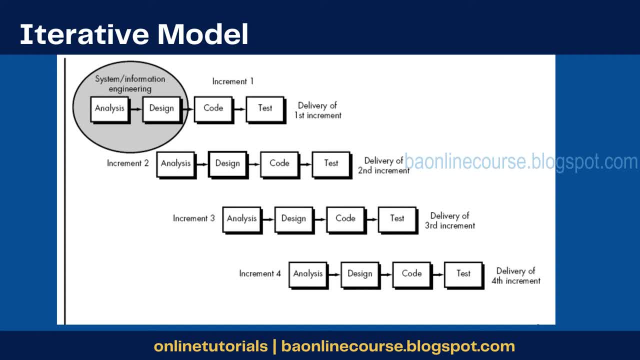 Mm-hmm. Oh, okay, So I think you know you can refer to the course content. I think it's comprehensively mentioned what all we would cover as part of that. All right, So guys, be on mute if you are not talking and then if you have a question, you know. 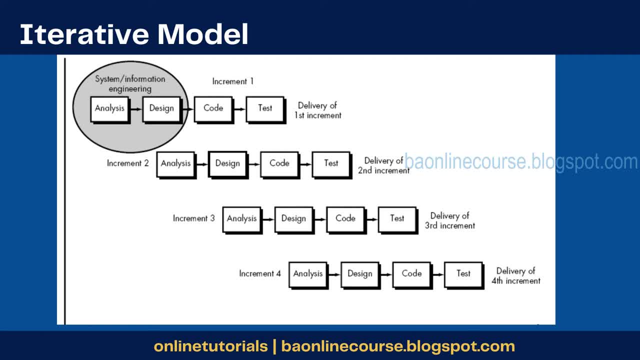 one request would be: you know, please keep the questions relevant to the. you know the topic right, So if the topic is relevant to the topic, ask them interrupt me. Otherwise, hold on your questions till the end of the session. 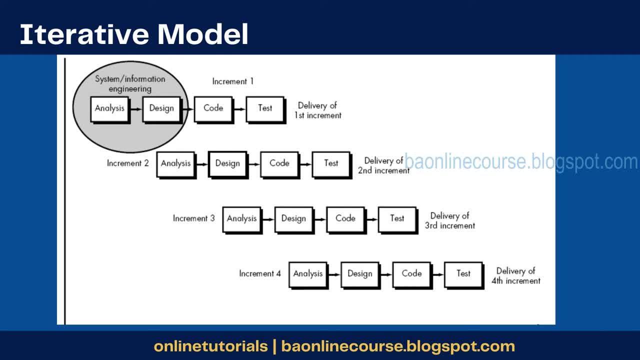 Once the session is complete, then we can take up your additional questions. Okay, So that way we'll be a lot more focused on the topic and we won't have too many disruptions. Okay, But feel free to interrupt me if you don't understand the particular topic that I'm explaining. 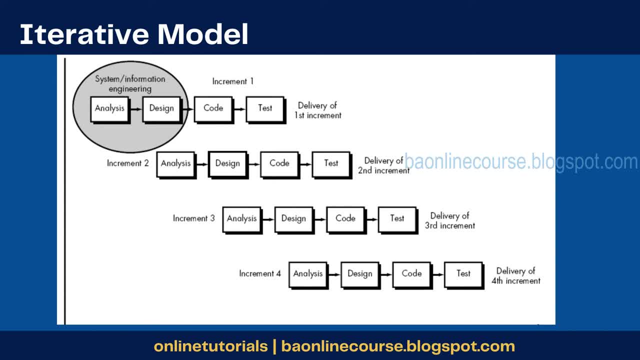 Or you want more details about it, or if you have a question regarding that, feel free to interrupt me. Okay, Right, So we are talking about the various types in which the projects could be executed, And iterative model is one of them. 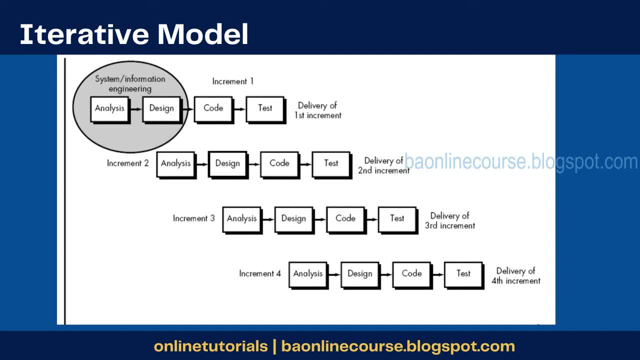 Now, generally we would go for iterative models where the project timelines are long, right? Let's say, a project typically would have taken you two years. Now that's too long a time for you. You have to wait till you start using the system, right? 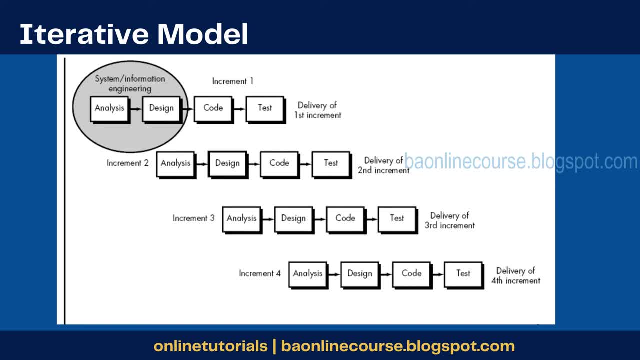 So by the time you know the system is developed, and then you are, you know good to go, you know use the system. Now the requirements could be outdated or the technology could be outdated, right? So you might not find much use of that system after two years, right? 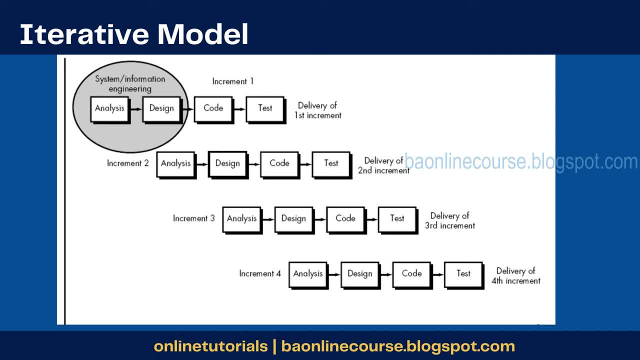 So you know, a lot of projects would tend to be like that. So how do you handle These kind of situations? Now, the easiest way is you would break it down into smaller sub-projects and then handle it right Now. a classic. a good example would be your. you know your softwares in your mobile phones, right? 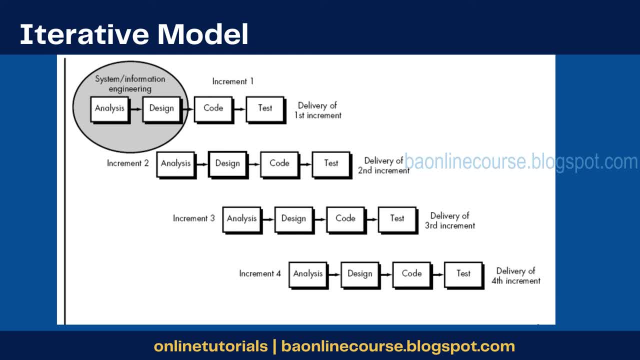 Now, if you look at it every three months or six months, you would have a version coming out, right? If you're using an Apple phone, there would be a- you know- iOS version coming in every six months, right? 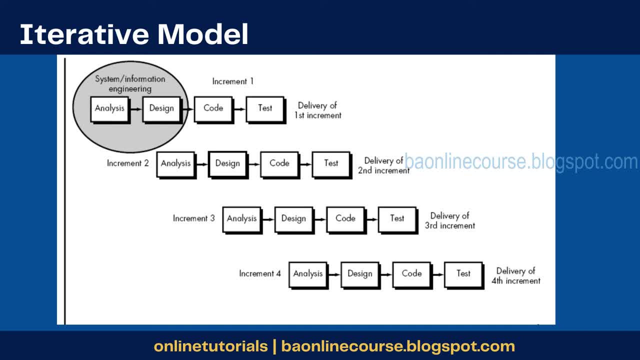 Now had these guys waited. They waited till they have this perfect version and then added all these features and then given to you. it might take- have taken them, like you know, some four, five years to complete that right. 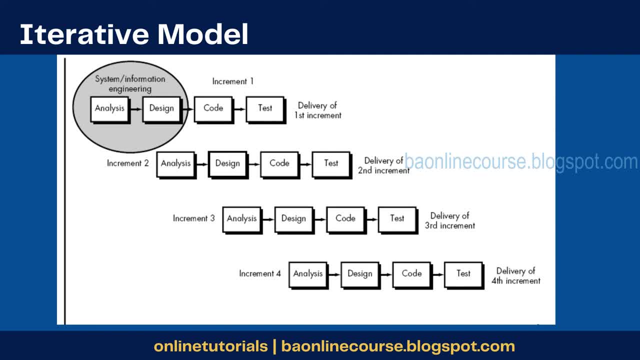 And they would have lost so much of business because of that. But what they did was they came up with the first version, maybe, you know, in 2005,, 2006,- with some basic features which could make the phone useful right. 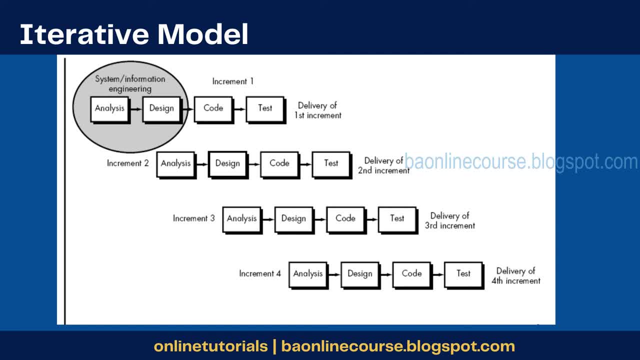 And people started using it And in the second version- iOS 2, they gave up, came up with multiple other additional features right. So incrementally, the functionality was delivered right Now. this way, they didn't have to wait till they have developed the product comprehensively and you know, the timelines were also reduced right. 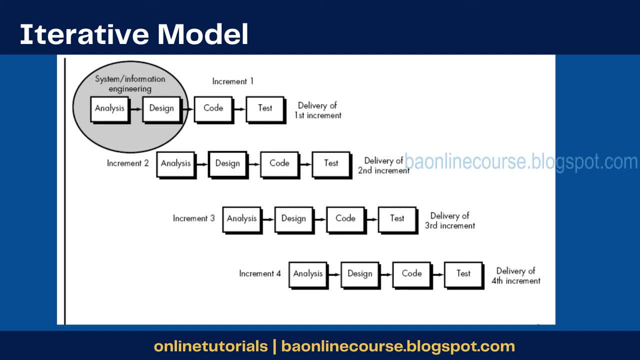 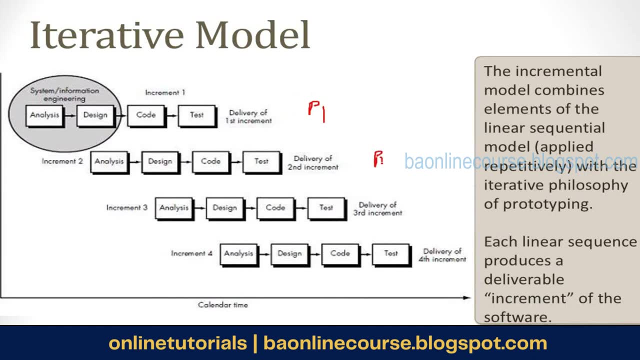 So, rather than wait some four years to deliver an iOS product, they did that within six months or so, right? So something like that. So you know you're breaking down a project into smaller phases, like phase one, phase two, phase three, right. 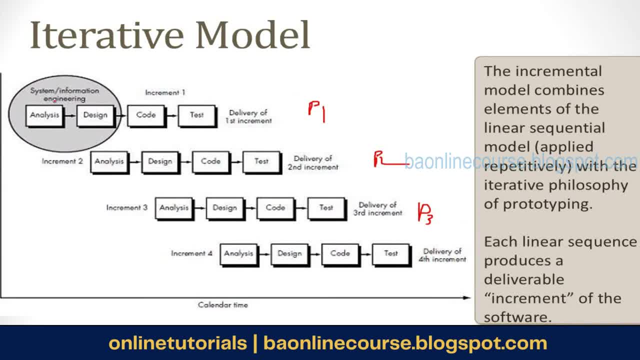 And each one of these phases would have some functionality within it, right? So if you have a scope, you're breaking down into, let's say, four subdivisions and saying this was phase one, phase two, Three and four, right? 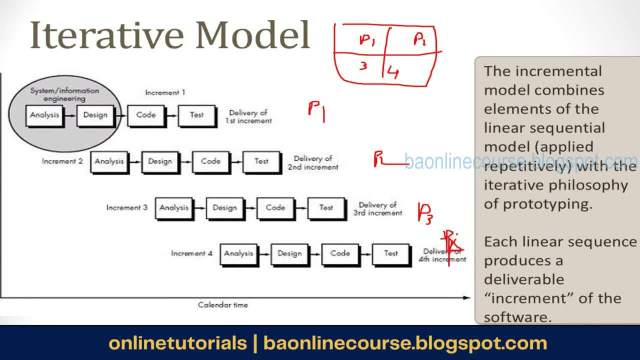 So in each of these four phases you'd have all the functionality covered, right, But you're giving it in each. you know each phase. you're considering it as a whole project and then delivering it, right. So you're doing your requirement analysis, design, development, testing and then delivering it to the end users, right? 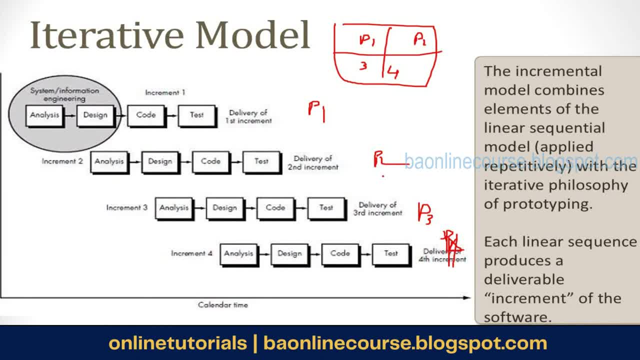 So while the users are using it, then your second implementation would start. okay, That's the advantage. You don't have to wait so long to start using the complete functionality. okay, So within each iteration. again, the steps are similar. 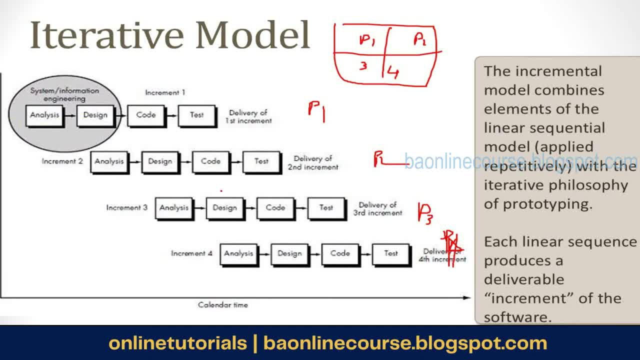 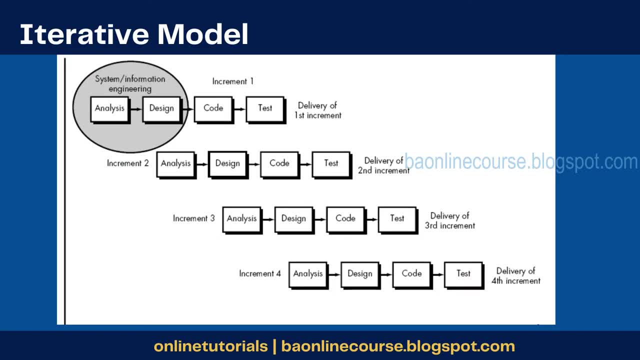 You would have an analysis, design, coding and testing happening. Yeah, Does somebody have a question? Okay, All right, So that's an iterative model. okay, Hello, This iterative model, is it similar to Agile? Not exactly. 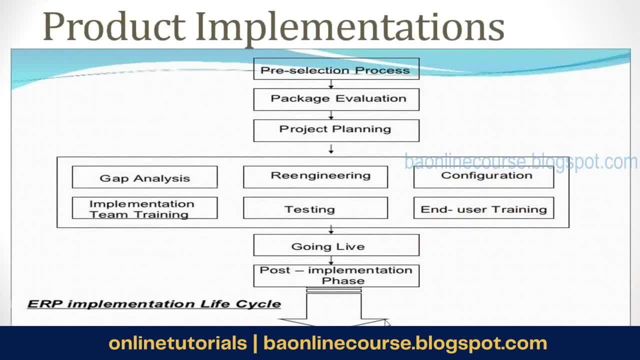 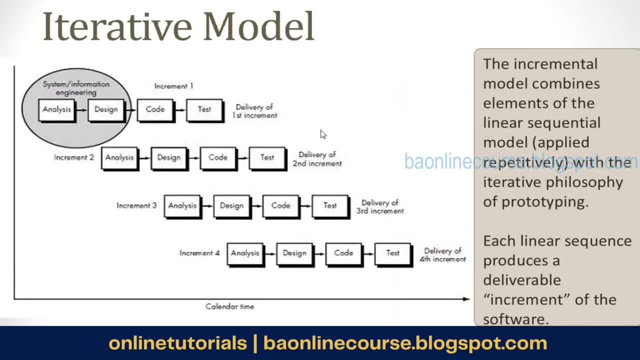 Agile works in a different way. I'll explain about Agile also later in this. Yeah, because in Agile also, like you know, they work on increments Right. So they would do that in Agile as well, But you know, this one would be done in a different way, okay. 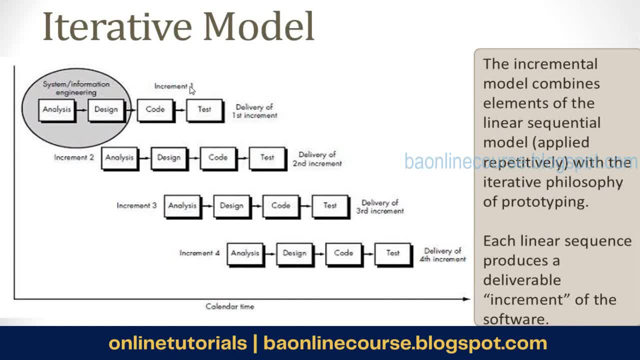 Okay, So, okay. So see, Agile works in a different way. I'll explain what is different in Agile. But iterative model, it's similar, like having multiple waterfall models within it, right? So there are four phases. You have broken down the requirement of the scope into four different phases. 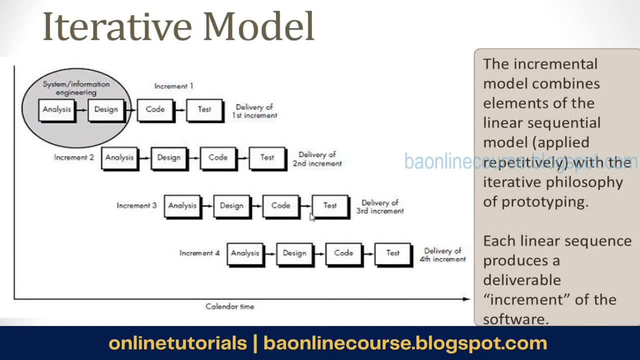 And each phase within it would be a waterfall in itself, okay, Okay. So when I come over to Agile, I'll explain the differences right. So the way, So the way the prioritization is done, or the way the you know the phases of the project. 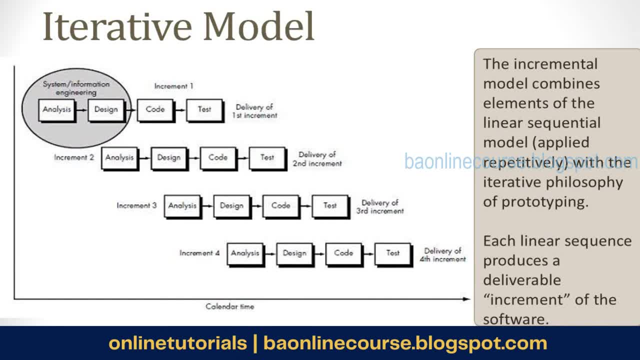 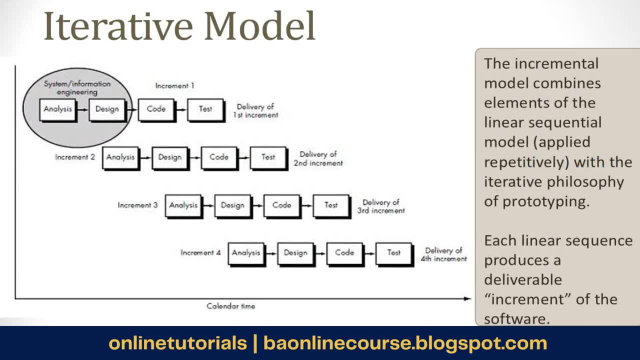 could be done. they would be very different The way that you communicate or document your requirements. all those details would be very much different from iterative model.